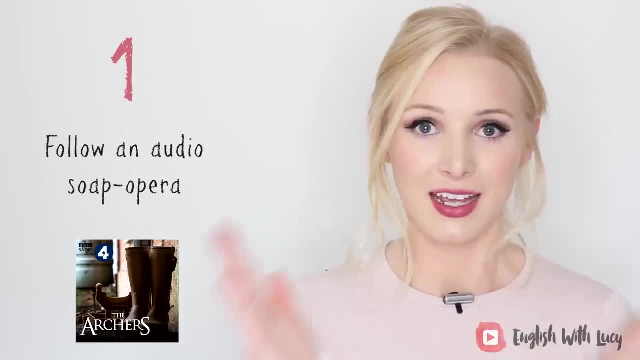 not least because it is the longest-running drama in history- It was started in 1950,, first aired in 1951, and also because I think it is absolutely perfect for English learners. It follows the daily lives and dramas of a group of fictional characters in the fictional countryside village of Ambridge. 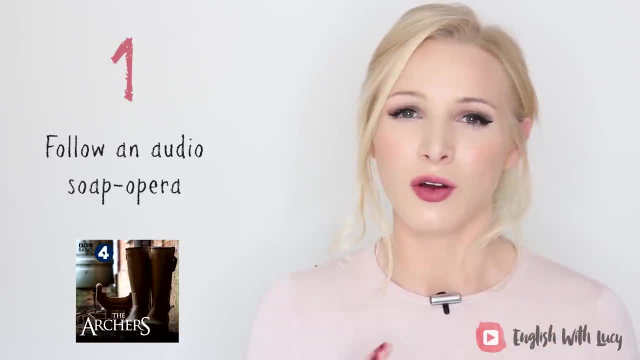 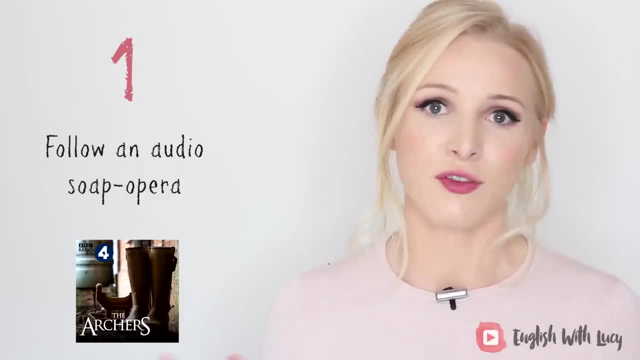 it's written in English and it's written in English and it's written in English and it's written in British, But it's made in a relatively clear English in a variety of British accents and sometimes not British accents as well other accents. But it's fantastic because the plot summaries. 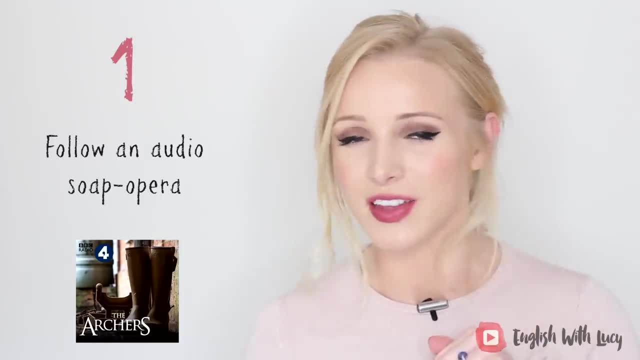 are posted on the BBC website. I will link to all of this below in the description box, And the great thing about this is that it deals with daily happenings, which is great for your life too- current events, routine things, and you can repeat all of the parts. 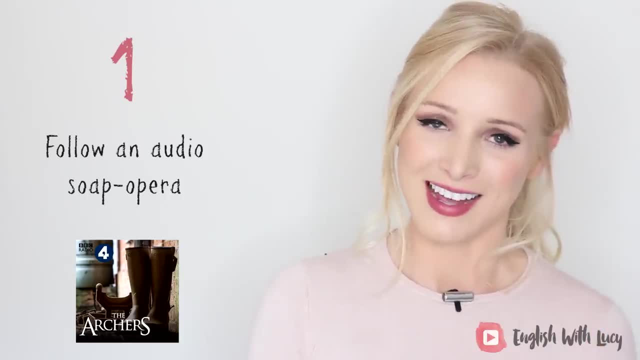 that you missed. It's on every single day, apart from Saturday, They have arrests- I- And once a week they condense all of the week's episode into one and that's called an omnibus And that's around 75 minutes long. 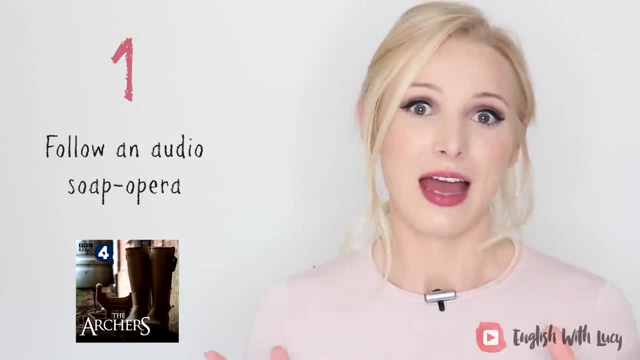 I love listening to The Archers when I go running. I listen to it every single day and if I miss one then I always catch up. There is no beginning and there is no finish to the series. There aren't any seasons, So it might take you a couple of episodes. 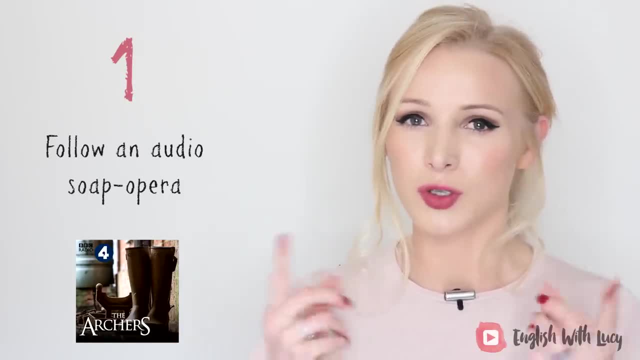 to get used to the storylines and to work out who is who and to recognise the different voices. Give it five or six episodes and you'll feel really included. It's wonderful because it's free to listen to, it's beautifully produced and there is a huge community of Archers fans. 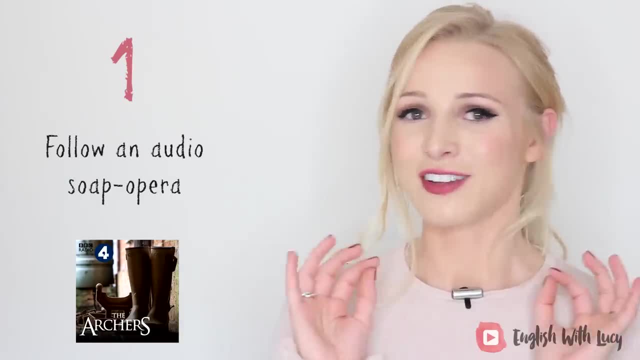 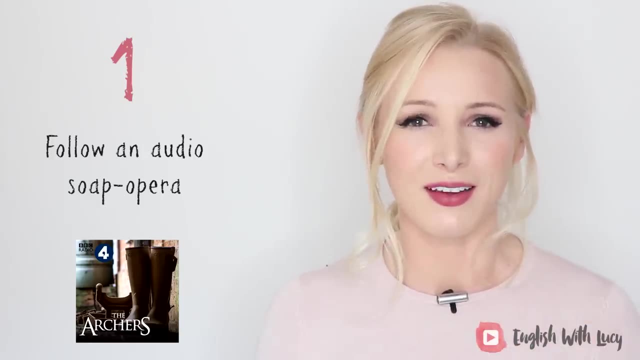 A lot of them are older, but a lot of them are younger too, And if you search hashtag The Archers on Twitter- big tip here- you'll see lots of people talking and discussing the topics of the episode and maybe you could interact with them. 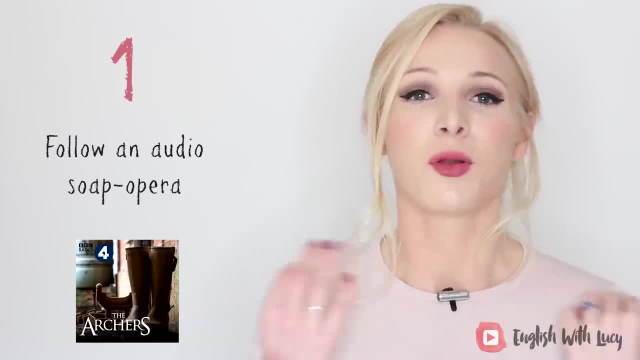 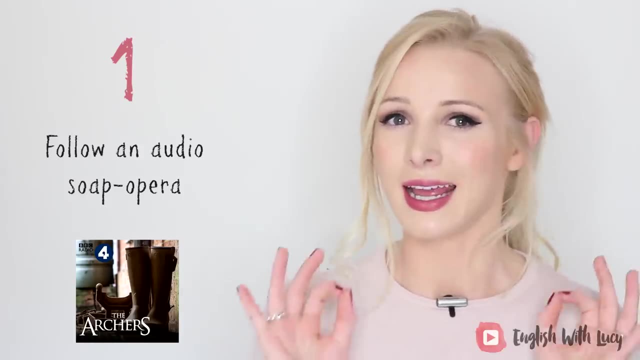 So I'm going to leave the links for The Archers episodes and also the plot summaries in the description box, And I really hope some of you take up this opportunity to listen to a daily English audio soap opera- 10 to 15 minutes every day. 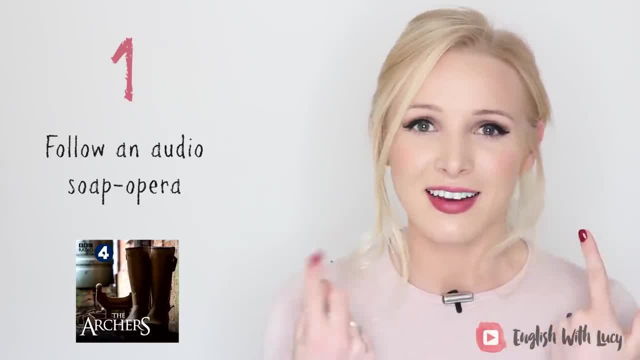 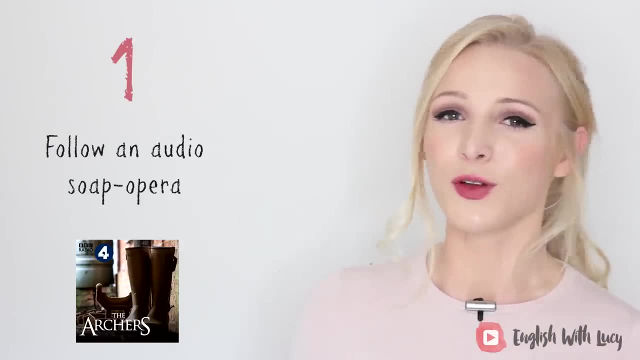 is definitely going to help your listening, It's going to help your pronunciation and it's just going to help your general enjoyment as well, because it's a great programme. Right before I get too passionate, let's move on to piece of advice number two. 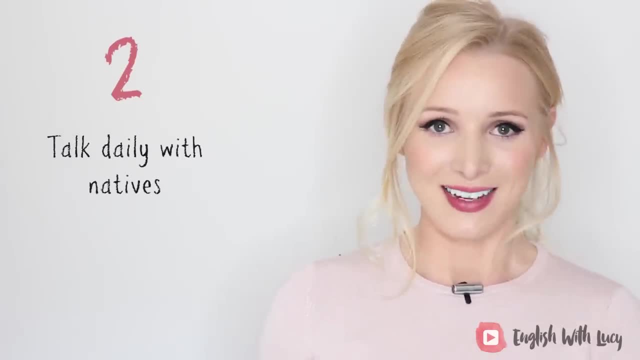 So number two is: talk daily with natives. Now I bet so many of you are thinking I wish I would love to talk to natives. I would love to talk to natives every day, but I don't know how and no one seems to want to talk to me. 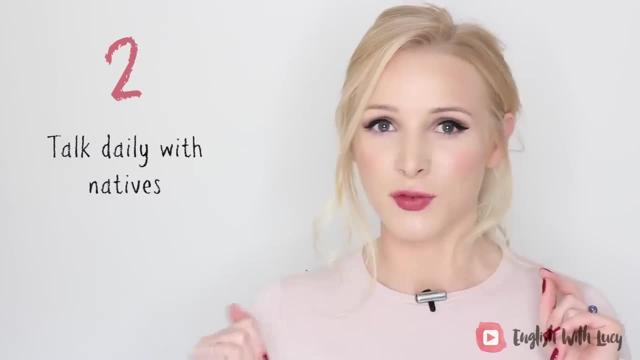 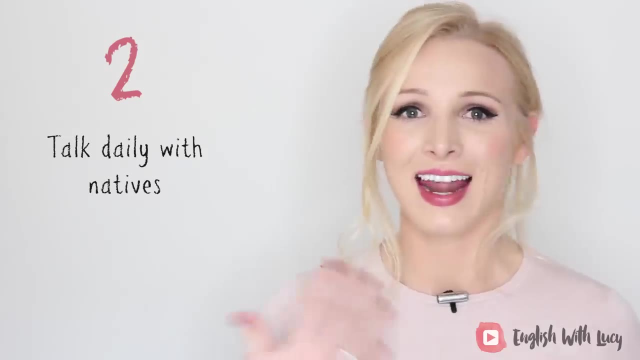 Well, I have a couple of suggestions. One is paid for and one is free, And the best thing, in my opinion, would be a combination of the two. So a combination of both paid for classes and language exchanges would be amazing, because you can take what you've learnt and heard. 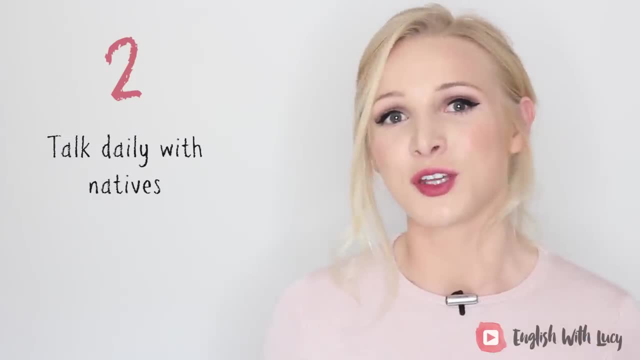 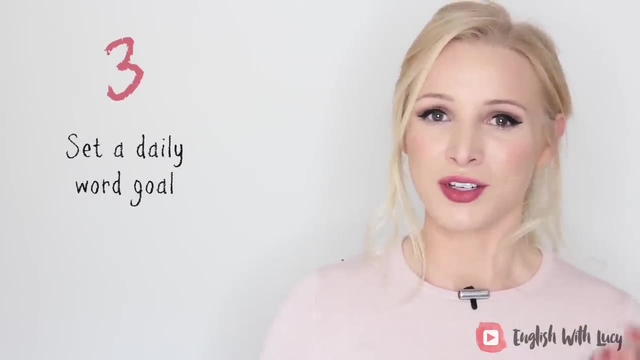 in the language exchange and verify it with your teacher for an extra layer of security to make sure that you're not making any mistakes. Now onto tip number three: a daily word goal. Learn X amount of words every single day. This tip is really important. 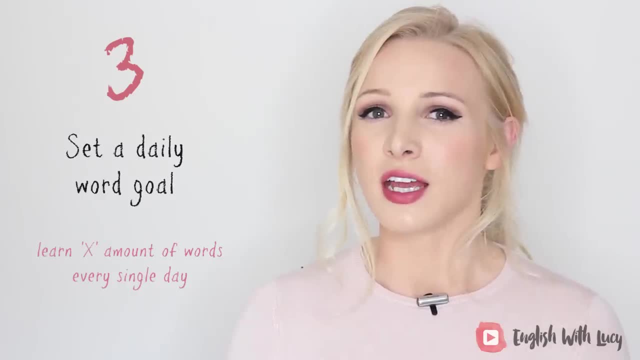 because it also links to tip number four. I have mentioned this strategy in a previous video, but I actually have a really important extra layer to this strategy that I would like to discuss with you. In order to build your vocabulary quickly, you need to learn at least one new word per day. 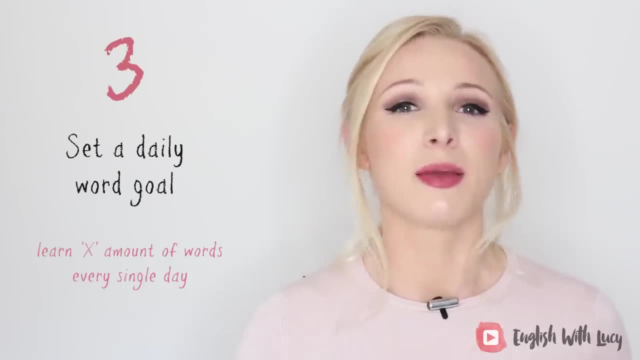 but hopefully more than that. I've spoken to you before about keeping a word diary or just a notebook or a list on your phone. Keep it with you all the time and always be aware, wherever you are. do I know that word in English? 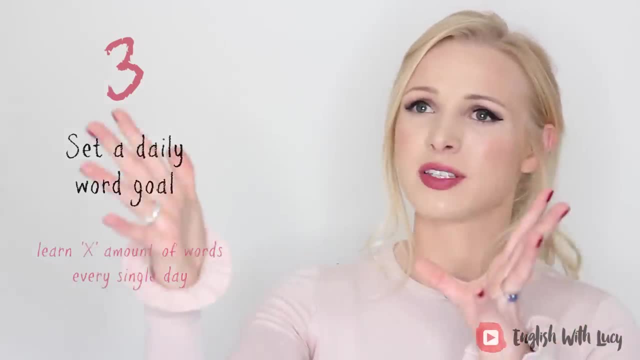 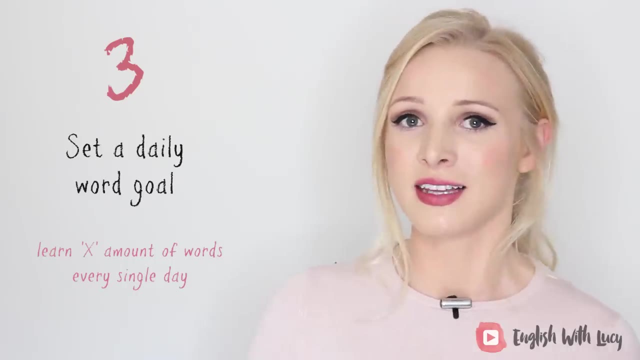 Do I know how to say that in English? You might see a tree. do I know how to say that specific variety of tree in English If you don't write it down in your own language in this book, in this list? 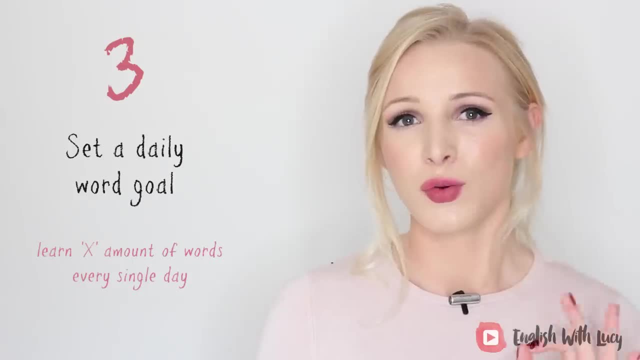 and then, at the end of the day, before you go to sleep, research all of these words and translate them into English. It will help you train your brain to always be hungry for English. After a few weeks, you'll be looking for new words that you can learn. 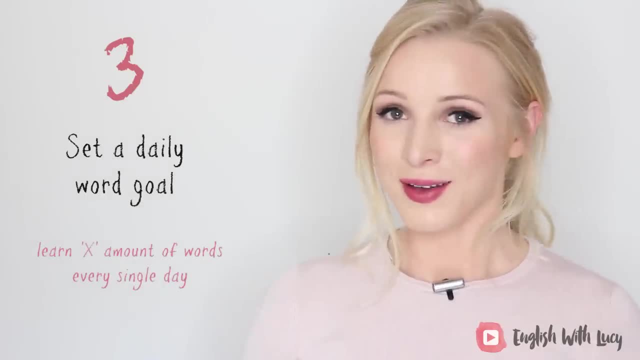 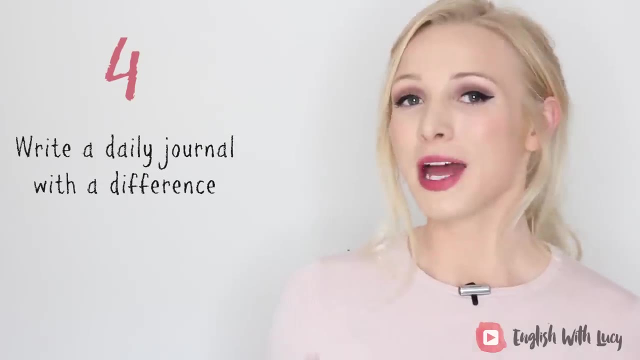 words that you didn't even realise, you didn't know. Now there is something else that you can do with these words, and this brings me on to point number four: Write a daily journal, with a difference Depending on your level: I would buy a paper journal or diary. 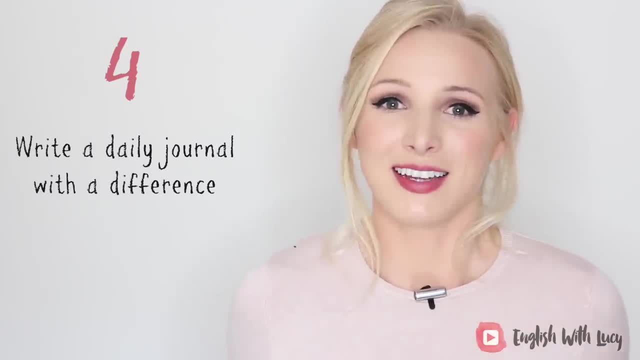 I get so tired in the evenings I can't spend loads and loads of time writing. so I personally would buy a work week planner or a homework planner or a study planner where you've got all seven days across two pages In each of those days. 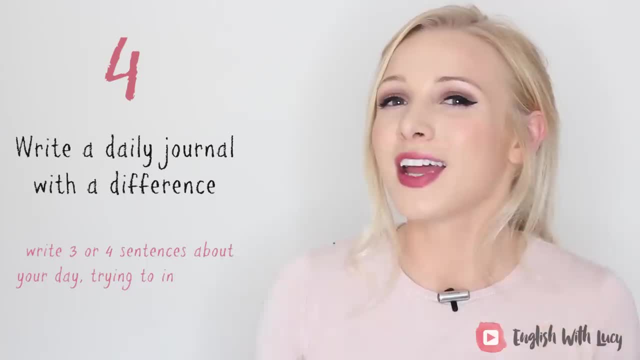 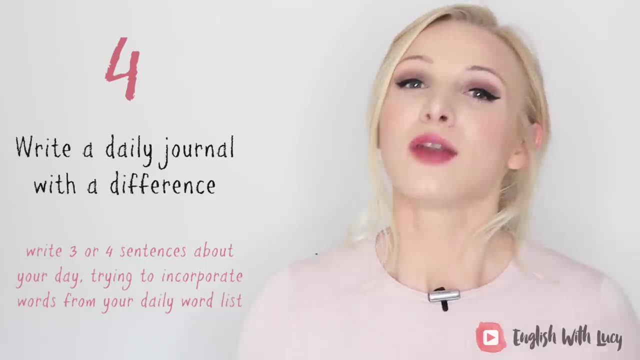 I would write three or four sentences about my day trying to incorporate those words that I learned in my daily word list- the words I mentioned in point three. That way, not only are you learning the new words and learning what they mean, but you're making sure they're fully integrated. 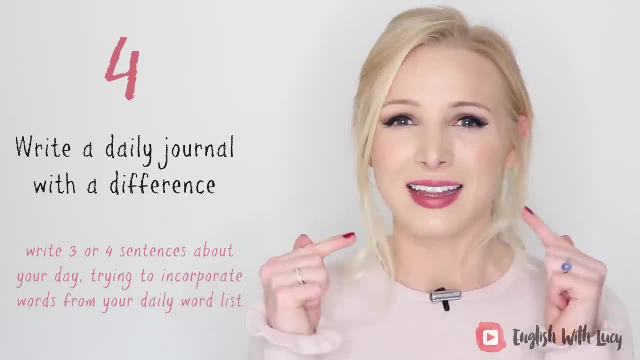 into your brain, and also, doing this before you go to sleep will mean they stick in there even more. Then you can wake up in the morning, read what you wrote the night before, and you've got those words fresh in your head, ready for the day ahead. 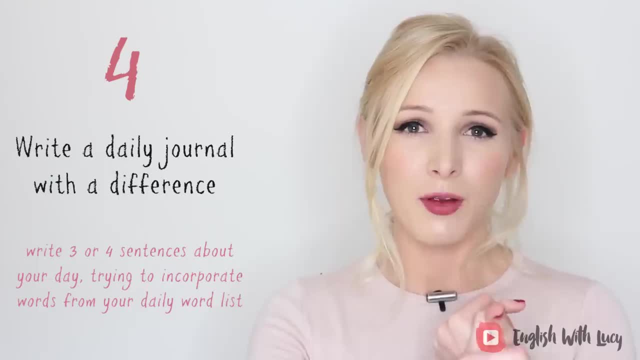 It's honestly such a fabulous technique because it builds your vocabulary, it improves your writing skills, it improves your reading skills. If you search the pronunciation of the word, it will improve your pronunciation and your listening skills, And if you book in sessions with language teachers. 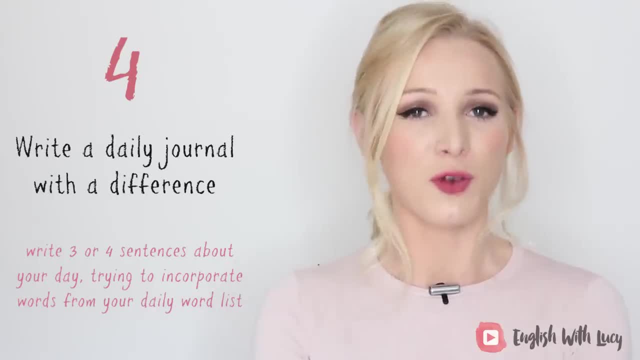 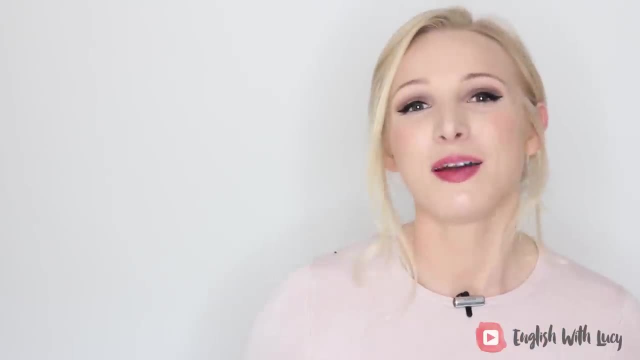 you can have them correct your writing. So every week you can bring them two fresh pages of writing for them to correct. Honestly, if you do this every day, it will help you so much. Right time for the last point, point number five. 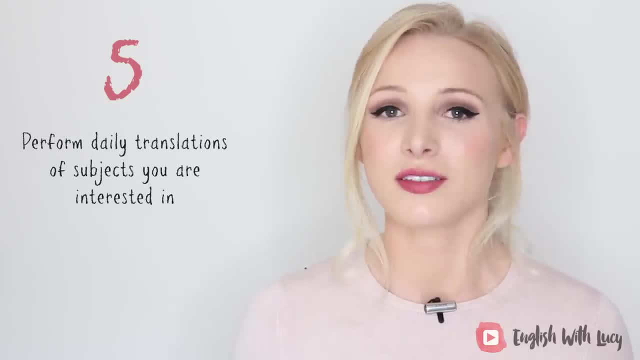 The tip is to perform daily translations of subjects you are interested in. Now, I know a lot of you want to stop translating and think in English. However, I think translation forms a very, very important part of language learning, especially when it's around something. 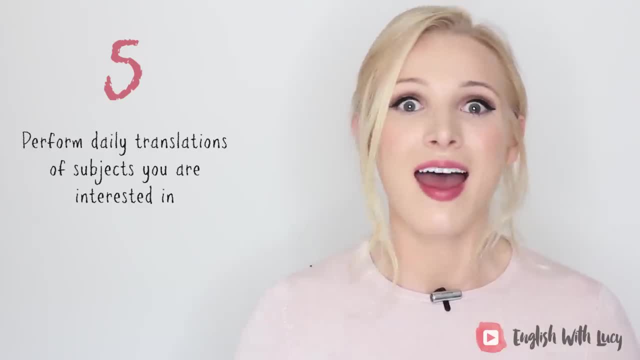 that you are interested in. It's really really good to compare how things are said in different languages, And translation helps you with that. In my opinion, the best way to practise your translation is absolutely free, which is fantastic, And it's right here on YouTube.